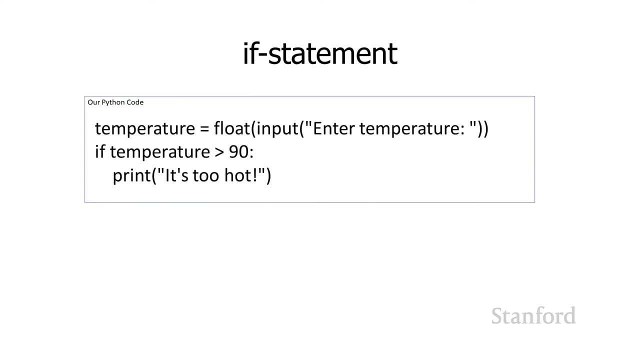 So let's take a look at our first control structure, which is the if statement. And so here's some code here with an if statement, And I'm going to be using temperature examples for today's lecture, So I'm going to go ahead and get a temperature from the user. 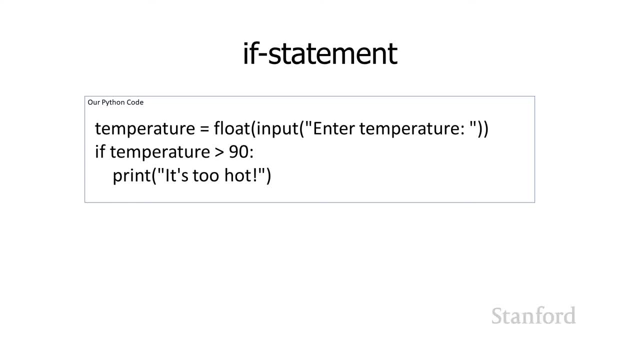 and then I'm going to have the computer give its opinion on what it thinks of this temperature. So this code pretty much. you could probably look at this code and figure out what it's doing. So it retrieves the temperature from the user using the input statement. 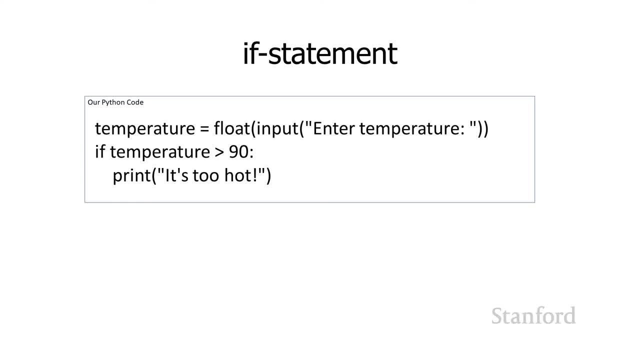 And then you'll recall. we need to convert that because generally the input statement is going to return a string which will be treated as text, And in this case we want to treat it as a number, And so we're going to convert it to a floating point number. 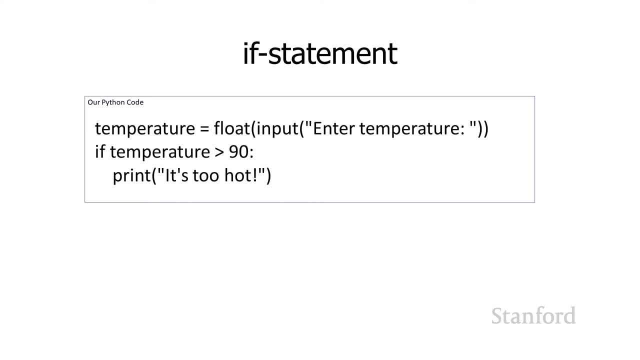 And then we're going to compare that floating point number which we are storing in the variable or storage location which we have named temperature, And if that temperature is greater than 90 degrees, we're going to print: it's too hot. 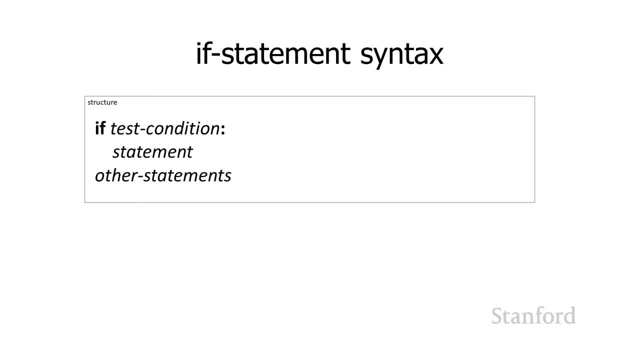 So let's take a look at the syntax of this if statement, And so you can see, here I've got the word if. This is what is sometimes referred to as a keyword. It is a word that has specific meaning. in Python, It's also sometimes referred to as a reserved word. 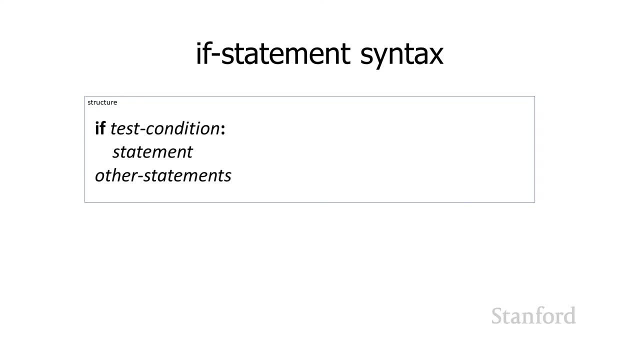 because you cannot name a variable. if So, if you were to name a variable, if the computer would get very confused. If you're familiar with the old comic routine- comedy routine- who's on first? that's the sort of situation you would get into. 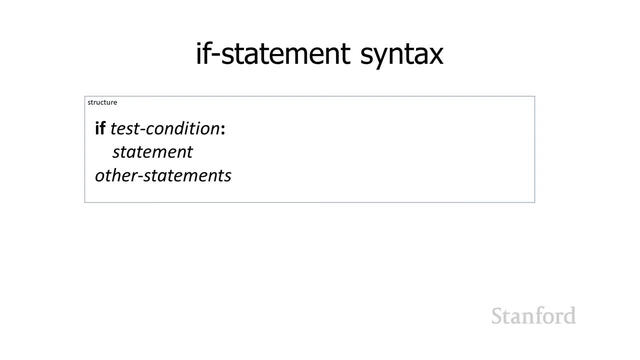 All right, so we're going to write down the word if, And then we're going to have some sort of a test condition, And I will take a look at the sorts of test conditions we can have a little bit later. We're going to follow that by a colon. 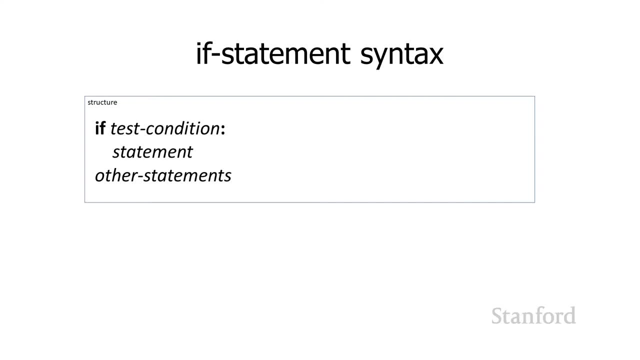 And then we are going to have an indented statement or set of statements, And then, after we're done with our indented statements, we are going to have some additional statements after that, Or we may have some additional statements after that, And so the way this works is the test condition. 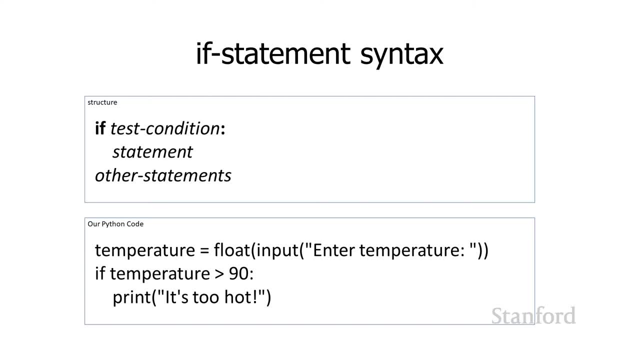 should give us a true, false value. We're going to take again, we're going to take a closer look at that in a minute- And so our test condition was if the temperature is greater than 90.. And if you think about temperature greater than 90,. 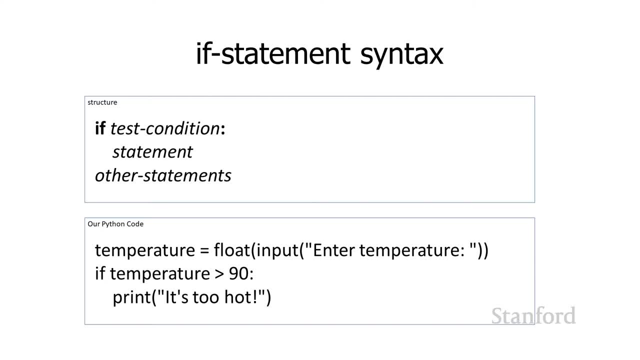 so either the temperature is greater than 90 or it's less than or equal to 90. So that's a true, false value. So either one could be true. OK, One condition is true or the other condition is true, And that's what we want for our test conditions. 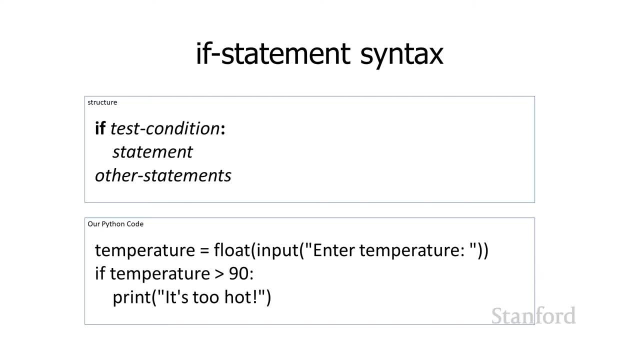 If that test condition is true- in fact the temperature is greater than 90, then what we're going to do is we're going to execute the statements that are indented below that if test condition, In our case it's going to do the print statement. 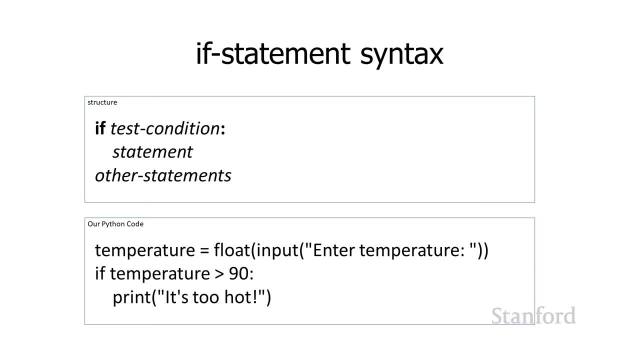 it's too hot, And then if we have additional statements that we want to always execute, those would go after the other statements. Let's take a look at a slightly more complex example. OK, So in this case I've got a number of statements. 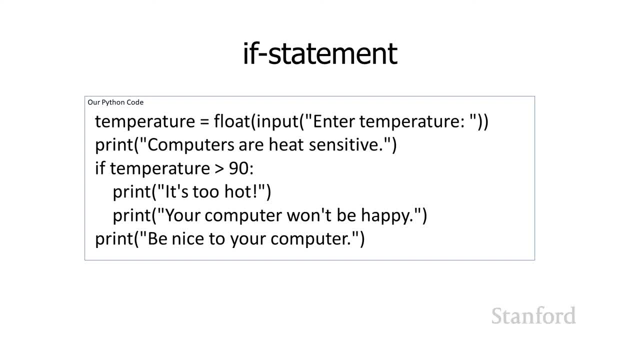 that get always executed. So essentially, the thing to be paying attention to is in Python, the indentation of the statements determines which statements are subordinate to other statements. So I've got that. temperature equals float input enter temperature. That always happens. The print computers are heat sensitive. 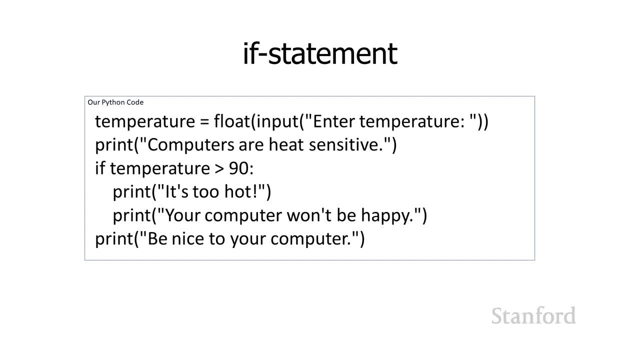 That always happens. The if temperature is greater than 90, that always happens. And then if we go all the way down to the bottom, the print- be nice to your computer. that also always happens. But those two intermediate statements, the print. 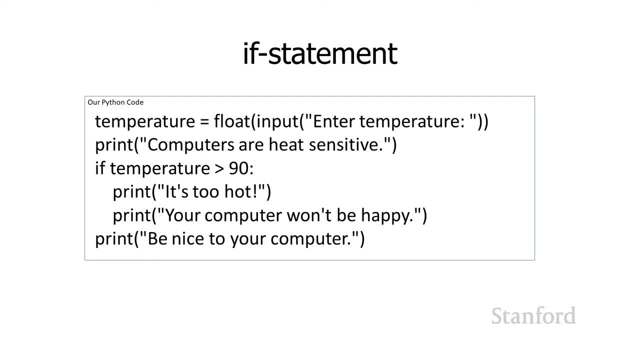 it's too hot and print your computer won't be happy. those are only going to occur if the test condition in our if statement, which is temperature is greater than 90, is true If the temperature is less than or equal to 90,. 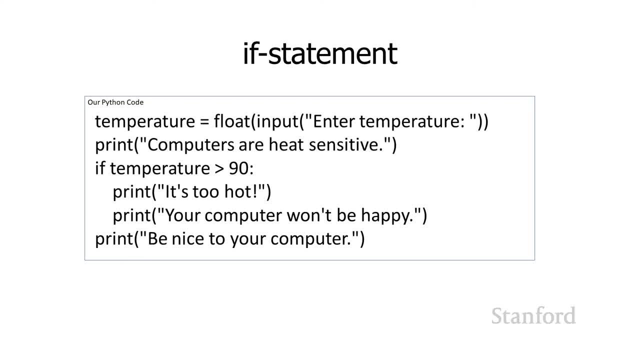 then those two print statements that are indented: the. it's too hot and your computer won't be happy. those will not be printed. So that's our if statement. OK, as I suggested earlier, sometimes there are times when we will want to execute one set of statements. 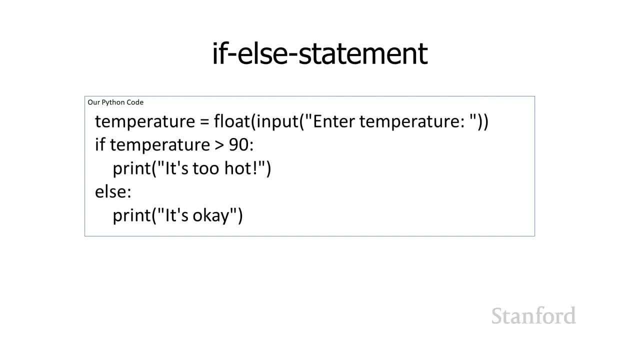 if a condition is true, and a second set of statements if the condition is false. And so that's what the if else variant of the if statement gives us, And so you can probably again look at this and figure out what it's doing. 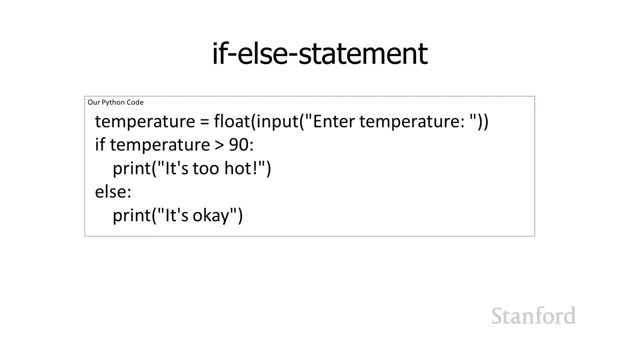 So again, we're going to get the temperature from the user And if the temperature is greater than 90, I'm going to say it's too hot And otherwise I'm going to print it's OK. And I should mention here I sort of briefly alluded- 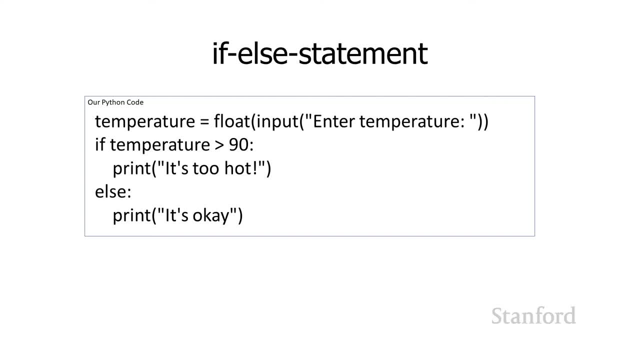 to this a little bit earlier, but let's talk about it explicitly. Notice that when you are doing a comparison like this, you need to think about if something is greater than something. you also need to think about if it's less than something. 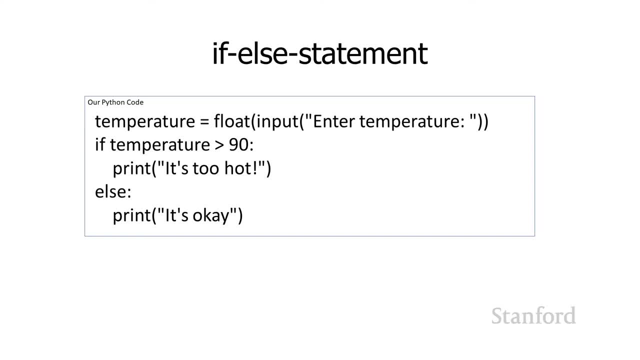 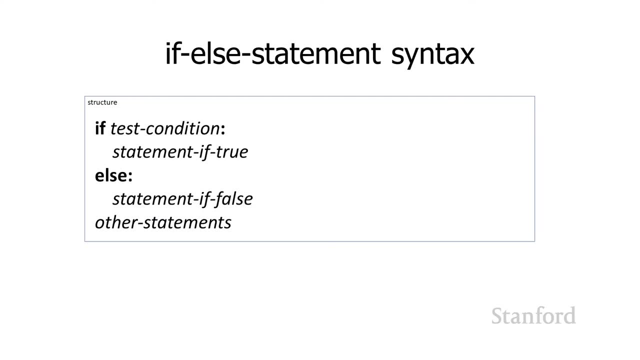 you also need to consider what's going to happen if it's equal to something. So in this case, if the temperature is exactly 90 degrees, I'm going to print it's OK. All right, Here's the syntax for our if else statement. 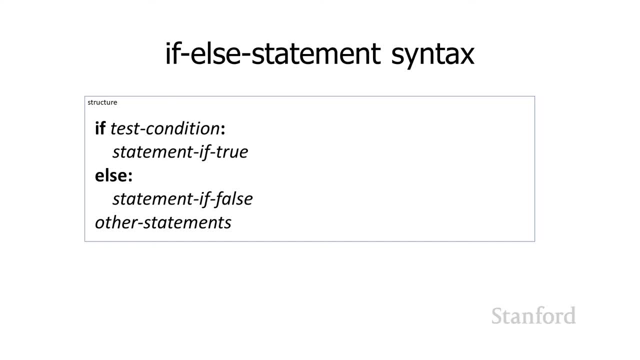 So I have if, followed by test condition, followed by colon. Don't forget that colon. That colon is super important. If you skip the colon, Python is going to be really unhappy with you and you have a syntax error and it's not going to run. 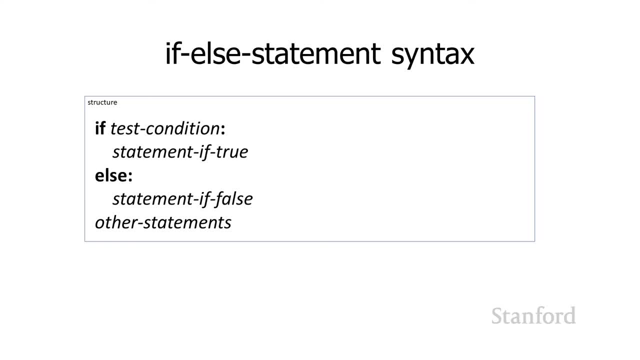 OK, If test condition: colon. and then I have that indentation, and then I have one or more statements that I want to carry out if the test condition is true. And so how does Python know which statements to execute? if the condition is true, It's whatever statements are indented after the if statement. 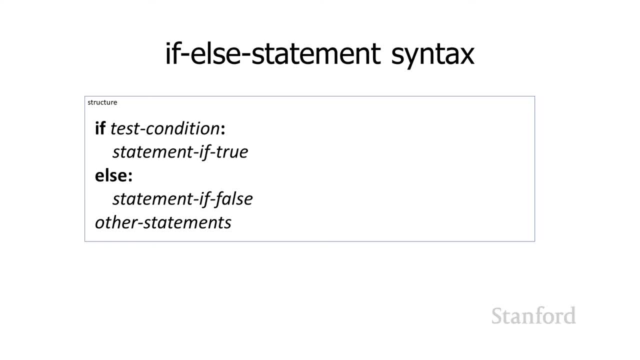 OK, then there's the else, And again there's a colon- there, Don't forget the colon. And then I have one or more statements indented after the else, And those will all get executed if the statement, if the test condition is false. 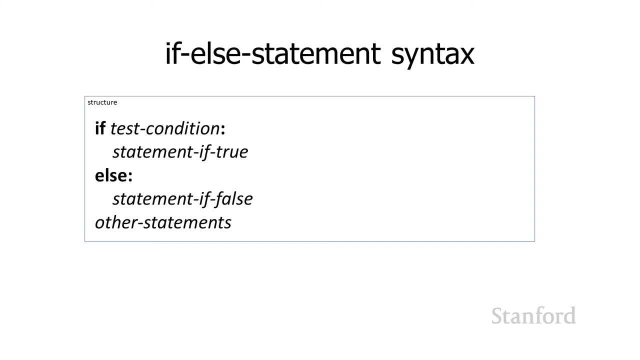 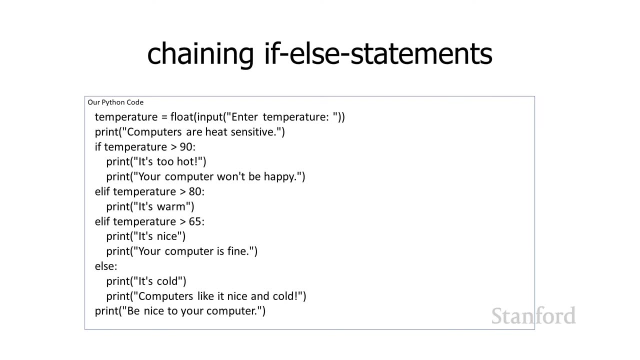 And then if I have additional statements which aren't indented, those will always get executed. I can also chain my if statements together. I don't think this has an official name, but I call them chaining if else statements. So you can see, in this case I'm checking. 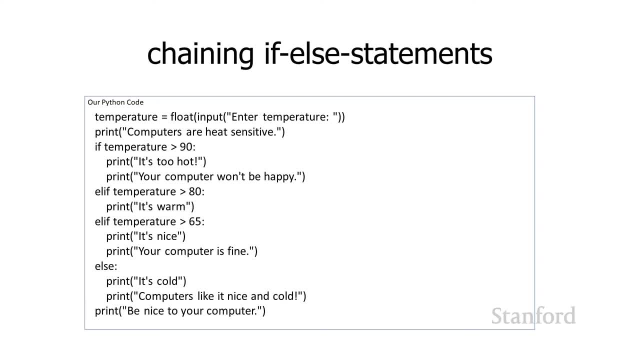 what the temperature is. I'm printing if computers are heat sensitive. I'm checking the temperature is greater than 90.. We've seen this before And then I have that l if temperature is greater than 80, l if temperature is greater than 65, else print it's cold. 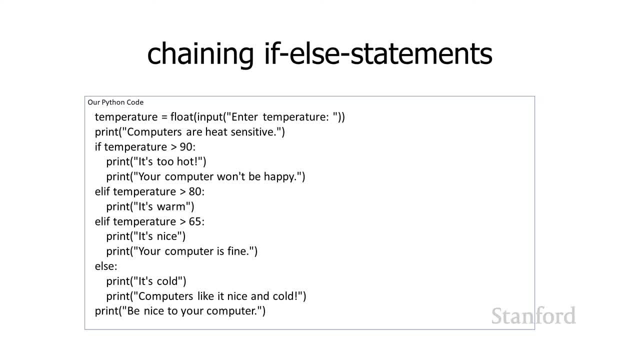 Computers like it, nice and cold, All right. so the idea here is it's going to try and carry out That temperature is greater than 90 comparison And if the temperature is greater than 90, it's going to go ahead and print. it's too hot. 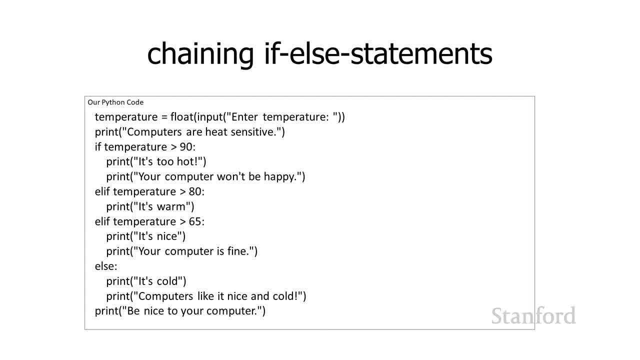 and your computer won't be happy. And then it will skip all the way down to the end print statement there. So the l? ifs, l ifs else will all get ignored, if that first test condition, temperature is greater than 90- is true. 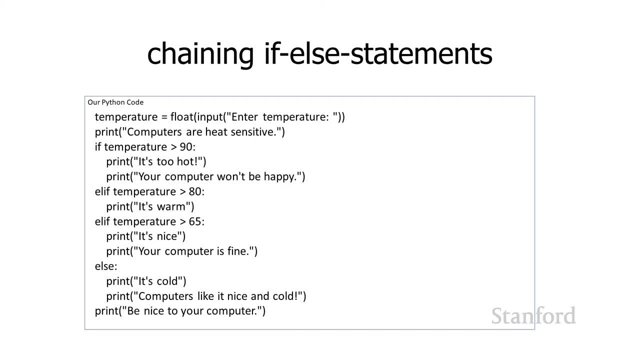 If temperature is less than or equal to 90, then it's going to do the test condition in that first l if Temperature is greater than 80. If that test condition is true, it's going to print it's warm And then, after it's done printing, it's warm. 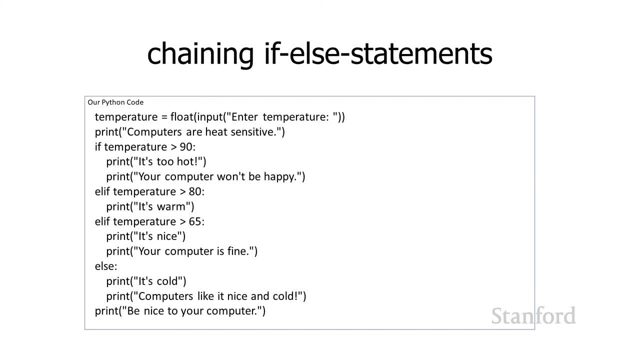 it's going to ignore the lf below it And it's going to ignore the else below it and go down all the way to print. be nice to your computer. If the temperature is less than or equal to 80, it's going to do the next test condition. 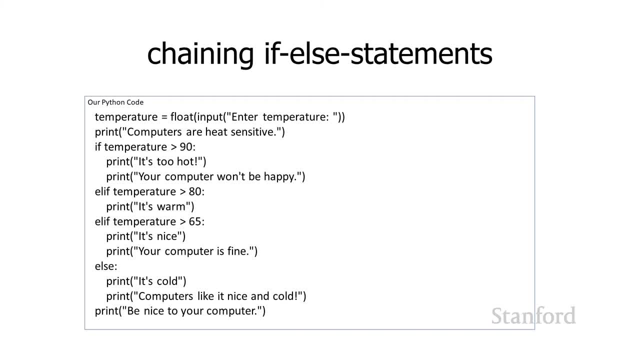 It's going to check whether or not the temperature is greater than 65. And if that test condition is true, it'll print: it's nice, Your computer is fine. And then it's going to skip the l statement and it will go directly to the print: be nice to your computer. 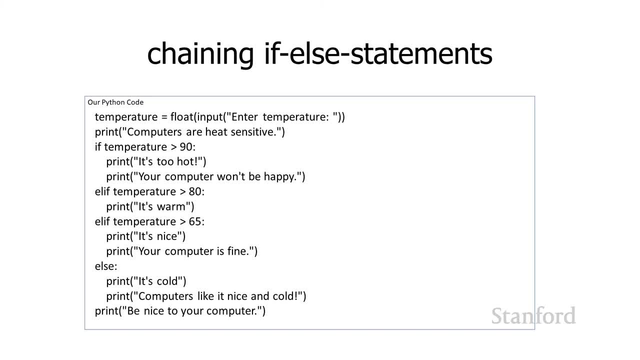 On the other hand, if the temperature is less than or equal to 65, it will print it's cold. Computers like it nice and cold And then it will always print: be nice to your computer. So it is possible to do this without chaining these together. 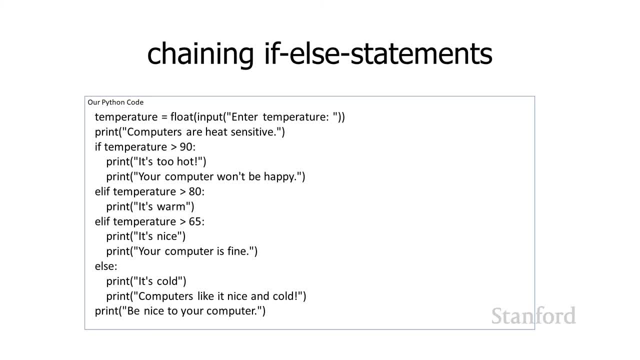 But it's going to be a lot messier because if I want to print- it's warm without the lf there- I'm going to have to both check that the temperature is greater than 80. But I'm also going to have to check that the temperature is in fact less than or equal to 90.. 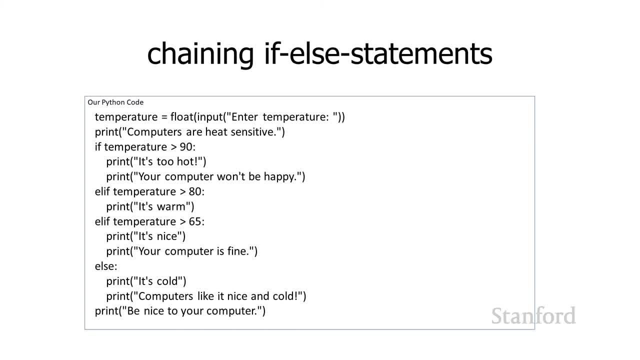 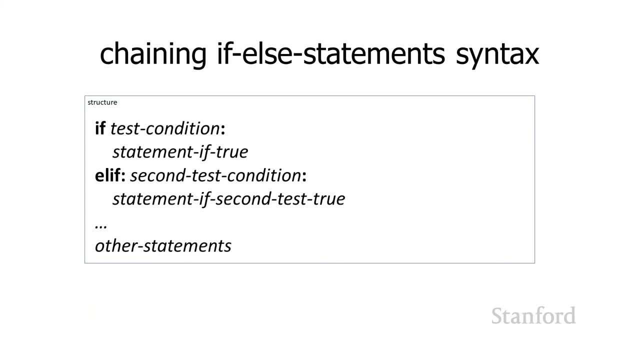 Because otherwise it's going to print both. it's too hot and it's warm, So these lf's are actually pretty handy, even though this syntax structure looks a lot, lot, messier. OK, so here's the general syntax structure for our chained lsif. 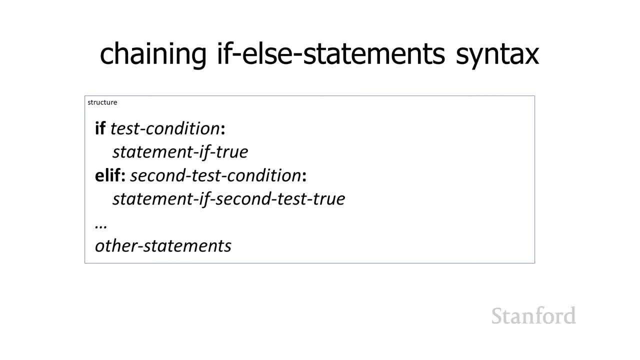 If, test condition, colon, and then a bunch of statements if it's true. And then, if that test condition is true, it jumps all the way to the end, after the if, after the lf. I don't have an else in this case. 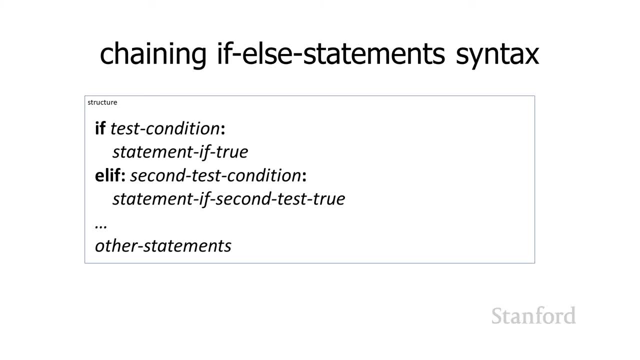 But if there were to end with an else, it would be after the else And that would go all the way down to other statements. If the test condition is false, it goes to the lf And it has a second test condition. If that second test condition is false, if I've got another lf, 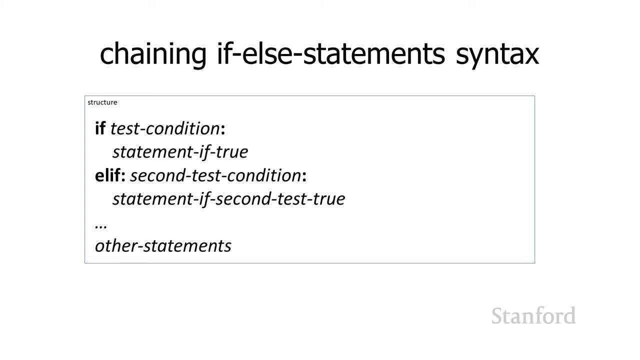 that third test condition would get checked. If there was another lf, that fourth test condition would get checked. And then you can either end with an lf, And if that last test condition is still false, none of the statements get executed, Or you can end this with an else. 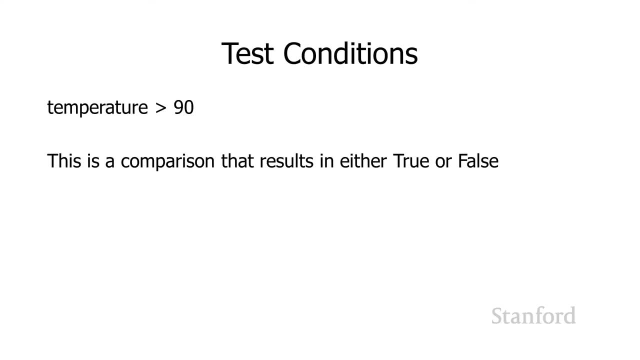 Either one works All right. let's take a look at those test conditions I mentioned earlier. So basically, what we want with our test condition is something that returns either a true or false value. So temperature is greater than 90. This is what we refer to as a comparison, or greater. 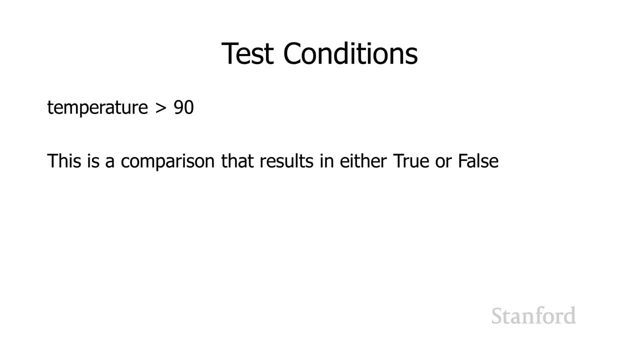 than as a comparison or comparator operator, And it results in a true or false value. A true or false value in computer science is often referred to as a Boolean value, And this is actually named after a person. There was a mathematician named George Boole. 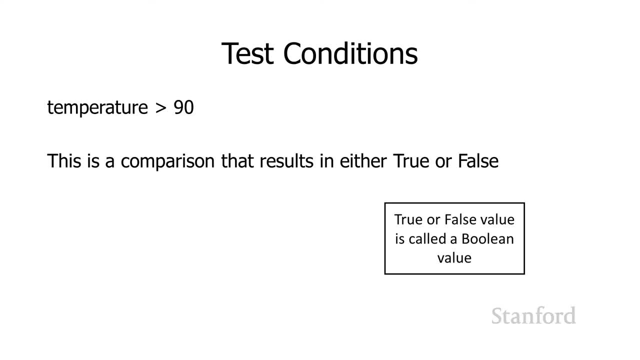 who came up with a set of mathematics based on true or false values. At the time it wasn't considered really important, But This was before we had computers, And now it's the basis of computing. So go, George Boole. Here are some test conditions you can use. 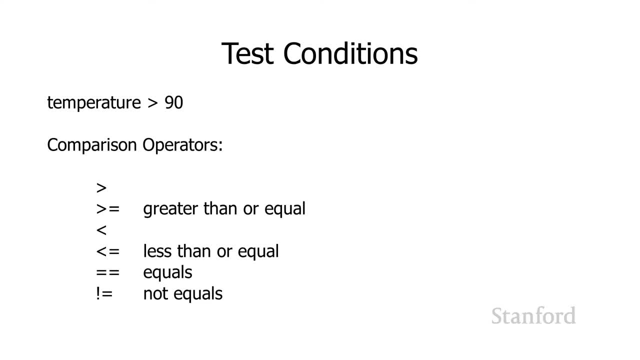 So there's the greater than I mentioned that you need to think about what happens when something is equal. So you can either say, hey, this is only true if it's greater, So temperature is greater than 90. Or you can be like, hey, I think, a temperature of 90. 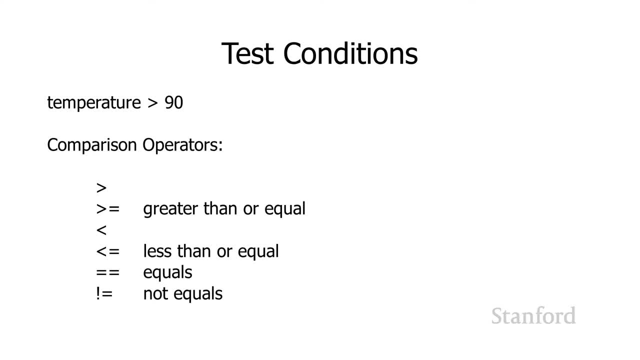 is pretty bad too. So, instead of using greater than, which says if the temperature is 90, that doesn't count, It's only if it's greater than 90. Or you can use the greater than or equal. Now, if you've seen mathematically, 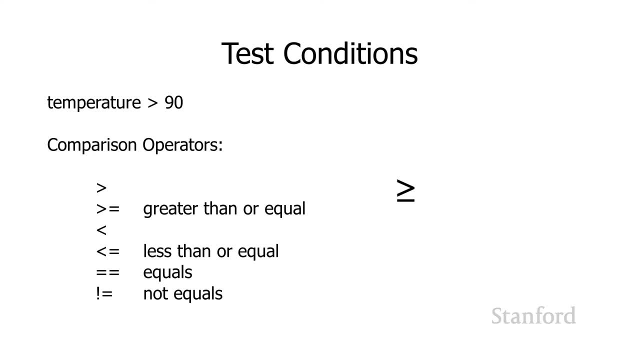 there is a greater than or equal, with the underscore under the greater than. We don't use that in computer science. Instead, we use the greater than sign, followed by the equal sign, because it's easier to type That greater than or equal to there's. 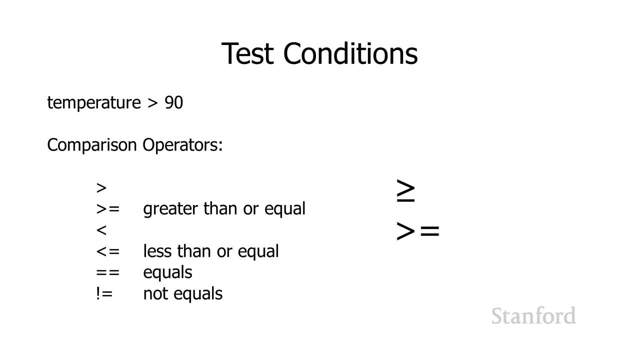 no way to type it on a standard keyboard. You have to do something special to get that going. There's less than. There's less than or equal. There's two equal signs, which means the two values are the same as each other. 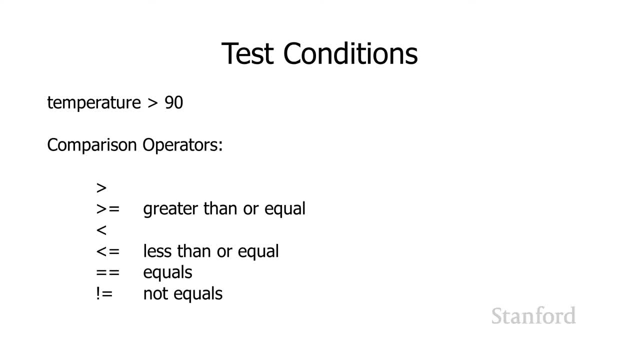 The single equal sign would be a variable assignment, and we don't want to do that. And then there's a not equals, which is created by using the exclamation point by an equals. This would be like: hey, I like any temperature. 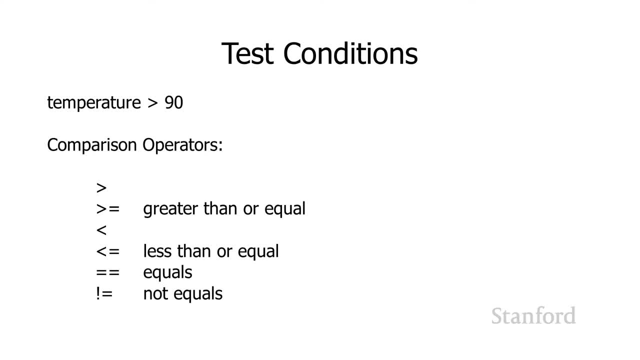 except for 80 degrees. If it's 81 degrees, that's great, If it's 79 degrees, that's great, But if it is equal to 80, that's a problem. So I would use the not equal to sort of signify that. 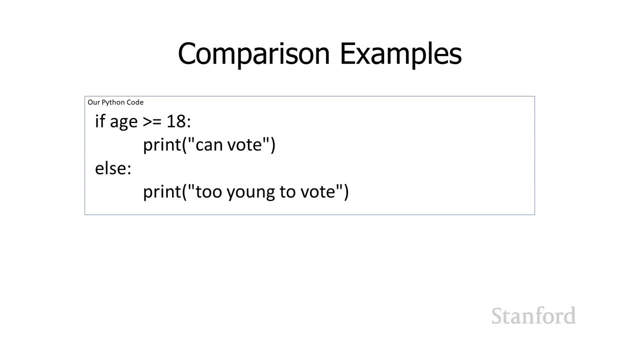 OK, So here's an example, a different example here, using one of the other comparison operators. So if age is greater than or equal to 18, then print, you can vote. Otherwise, print, you're too young to vote. Now we can combine these together. 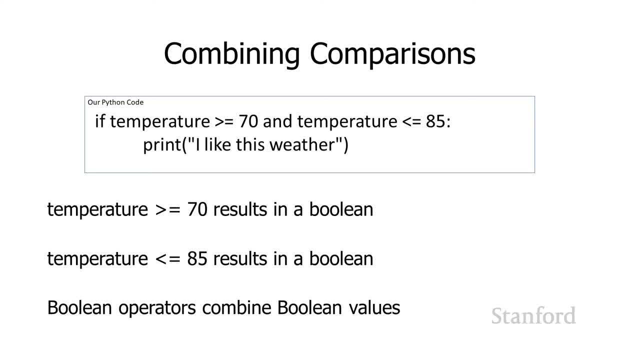 This does get a little bit messy, so you do need to be careful when you're using these, but they can be quite handy. So if I wanted to check that the temperature is between the range of 70 and 85, I can do that by clicking. 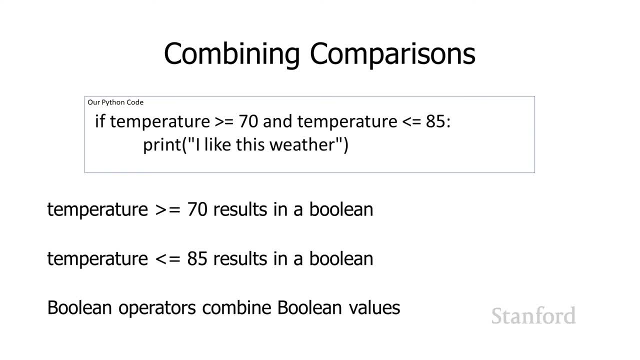 Combining two comparisons: I can compare the temperature and make sure it's greater than or equal to 70. And I can also compare the temperature and make sure it's less than or equal to 85.. And so I'm combining these together with an and. 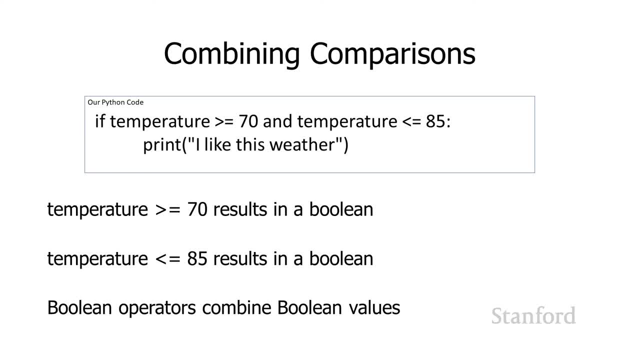 This is only going to be true. this print- I like this weather- is only going to get printed if the temperature is both greater than or equal to 70, and it is also less than or equal to 85. This is what I would refer to as a Boolean operator. 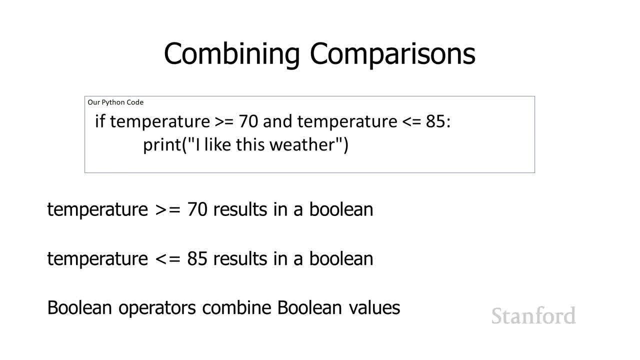 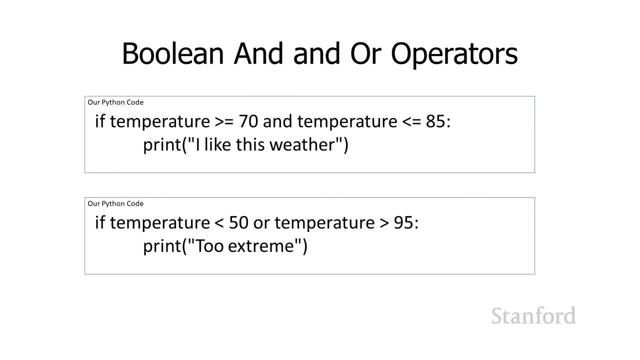 because it combines two Boolean values. Remember our true false value. These are things that result in true false values. They're just called Boolean values. There's also or operators. So in the second example here I've got an or. I say if the temperature is less than 50. 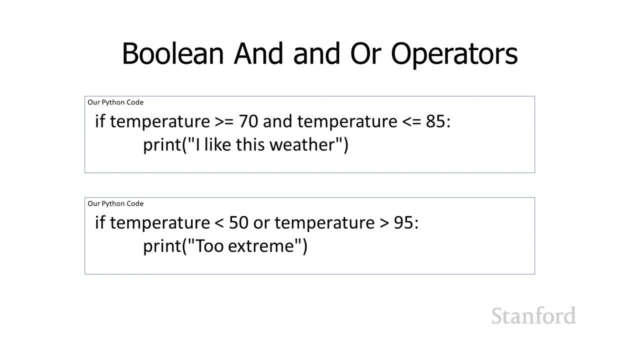 or if the temperature is greater than 95, then print two extremes. So my or operator is going to work if either one of the test conditions is true. So either the temperature is less than 50 or if the temperature is greater than 95,. 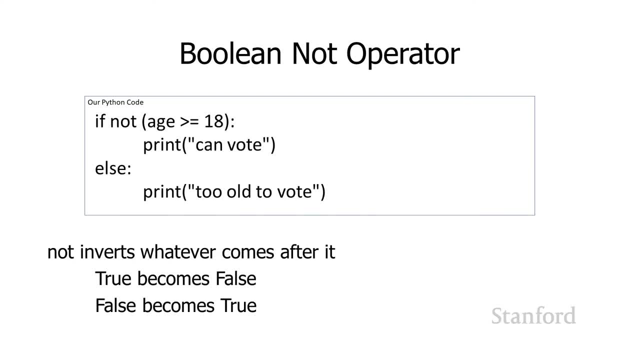 then the whole thing will be true and we will print two extreme. There's also not operator. It's a little bit, it's probably used a bit less frequently and it's probably a bit harder to understand, But basically it takes whatever, comes after it and inverts it. 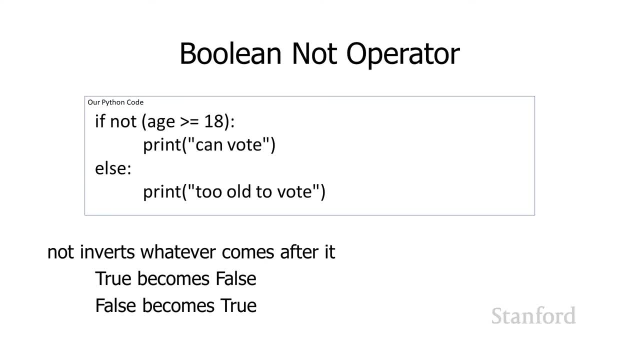 So before we had, if the age is greater than or equal to 18, people could vote. and maybe people are looking at the results of our previous election and thinking that, hey, I don't think we did so good with people greater than or equal to 18. 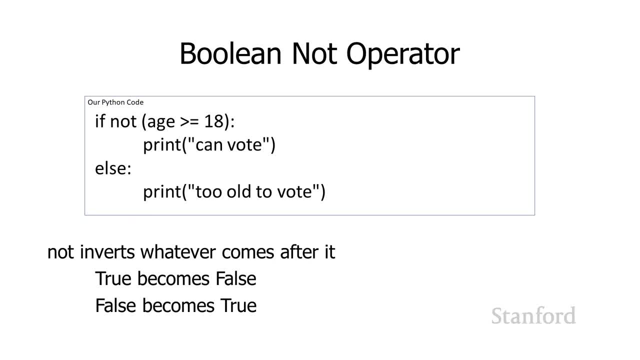 voting. So maybe we're just going to invert that. So we're going to say: if not, age is greater than 18, and so we'll have three-year-olds voting, And so if not, age is greater than or equal to 18,. 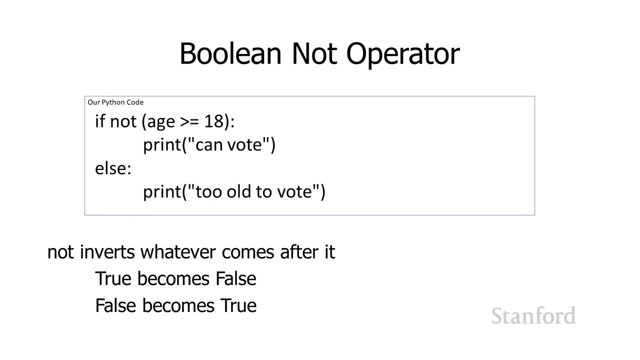 this essentially means that if the age is 18 or over, that comparison age greater than or equal to 18 is true, but the not actually reverses that. So basically, if somebody is 17.9, they would be able to vote. 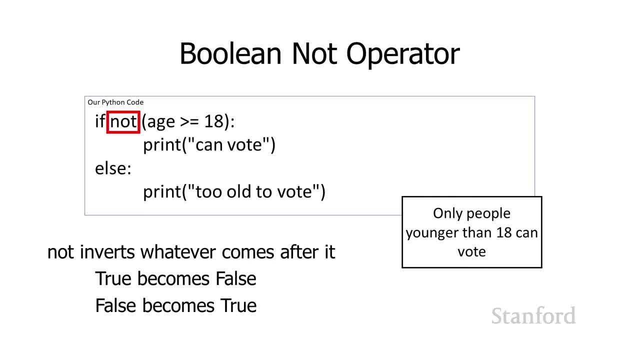 If people were 16,, they would be able to vote. If they were three, they would be able to vote. But if they're 18,, 19,, 20,, 50,, 70, they couldn't vote. All right, it's also possible to just put a Boolean value. 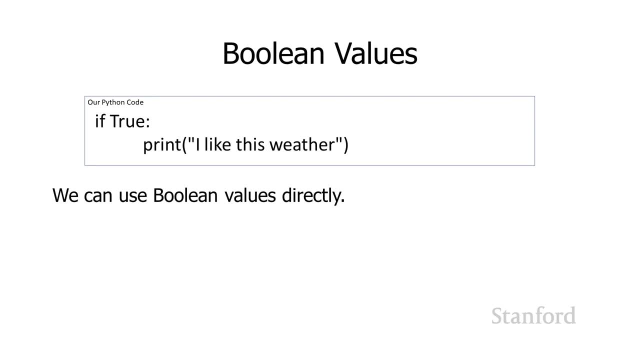 straight there So we can write Boolean values as true and false, And in Python these are written with a capital T. So if true, print I like this weather. This actually always prints I like this weather. You wouldn't use this. 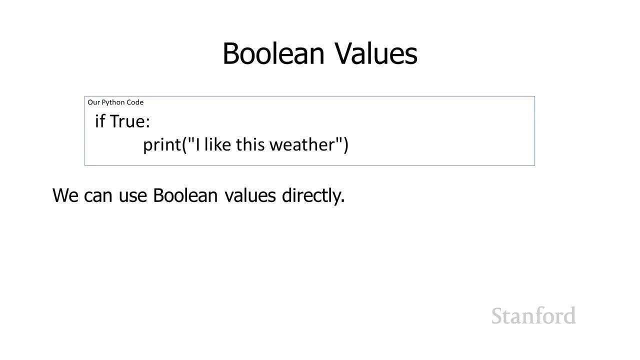 It's in an if statement, but there are some other control structures where some people do like using this particular method of always putting a true value there. I personally think it's a little odd. I do know there are reasons why they do it. 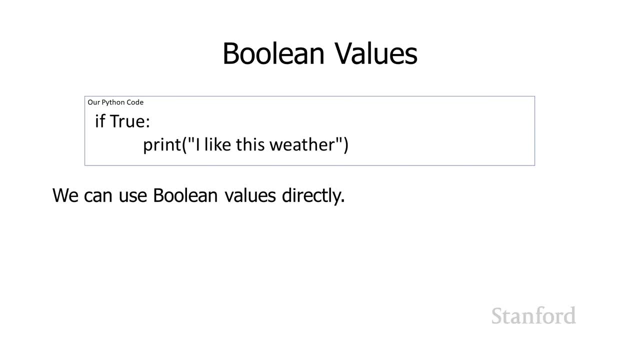 but you will see the sort of code. You won't see it with an if statement. So again, I've just written a Boolean value there directly and so this is always going to be true and so it's always going to print. I like this weather. 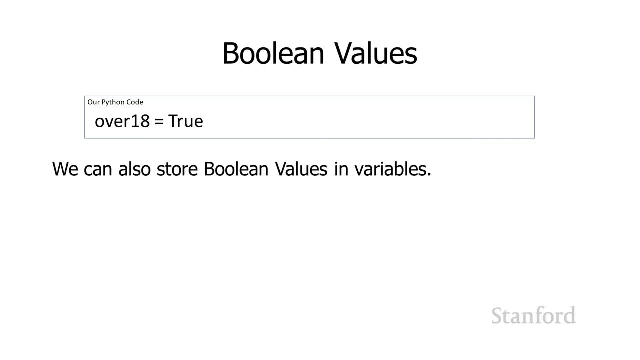 And you can also take these Boolean values and just store them into variables directly. So we've previously talked about how there are integer values, there are floating point values and there are strings, And it turns out Boolean is yet another type of value that we can store in a variable that we can assign. 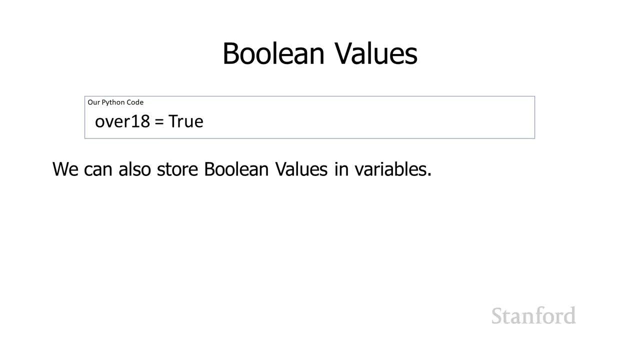 into variables, that we have operators that operate on them. just the same way, we have integers that we can store into variables We can use in operators. We can add and subtract them and so on, And so we'll see more of these in the next couple of weeks.